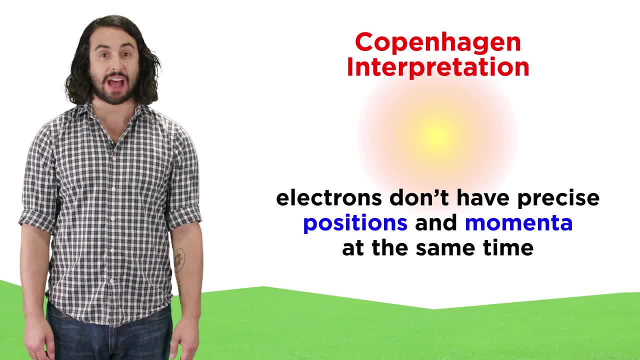 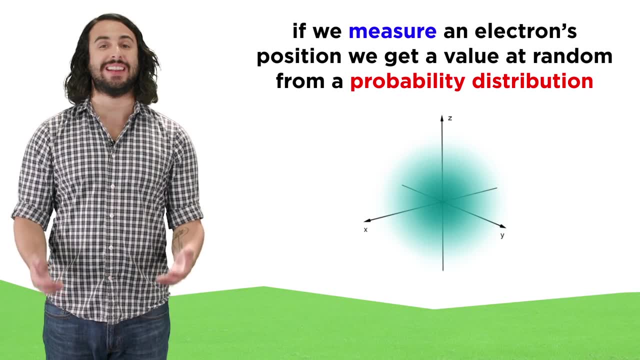 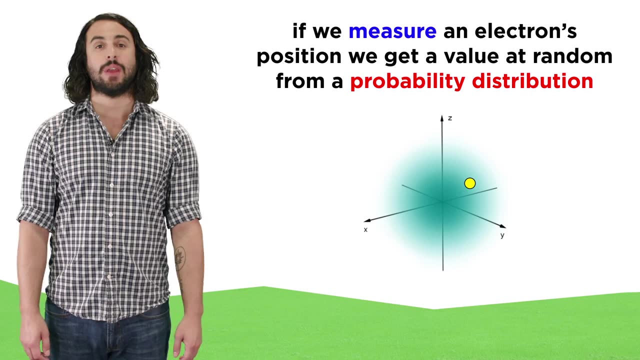 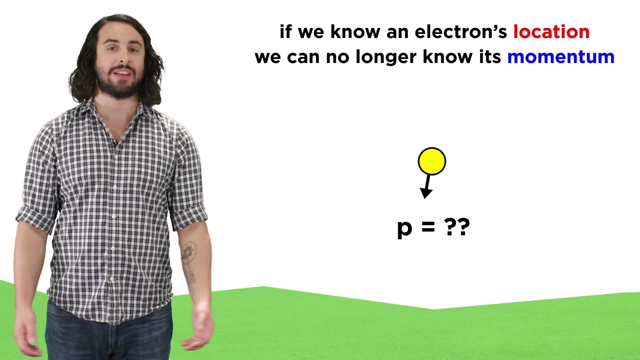 precise values for both of these parameters at the same time. So when we take a measurement, the result is randomly drawn from a probability distribution. An electron will seem to be in a particular location if, and only if, we measure its location. However, if we know its location, we can no longer know its precise momentum or what. 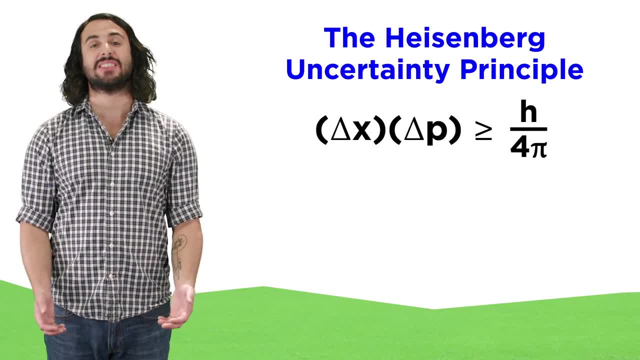 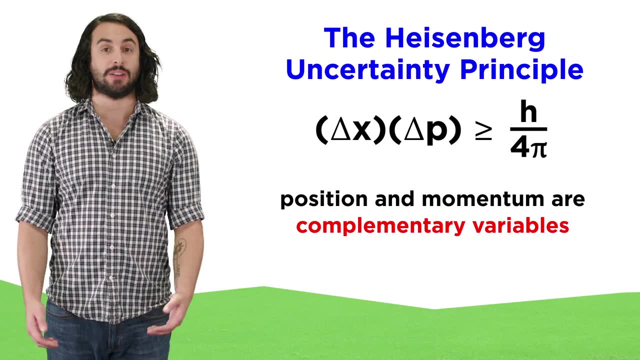 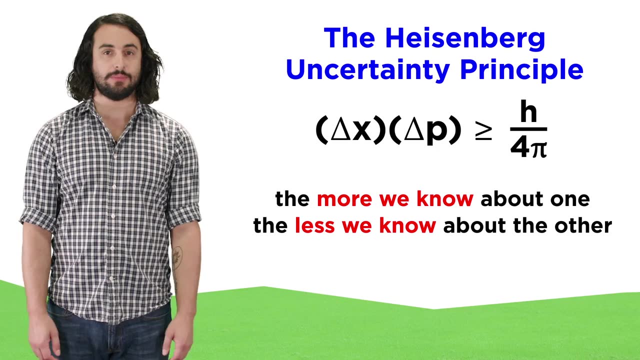 it's doing, and this notion is summarized in Heisenberg's uncertainty principle. This states that when looking at complementary variables like position and momentum, the more precisely one parameter is known, the less we know about the other. Here, delta X represents the uncertainty in position, while delta P is the uncertainty. 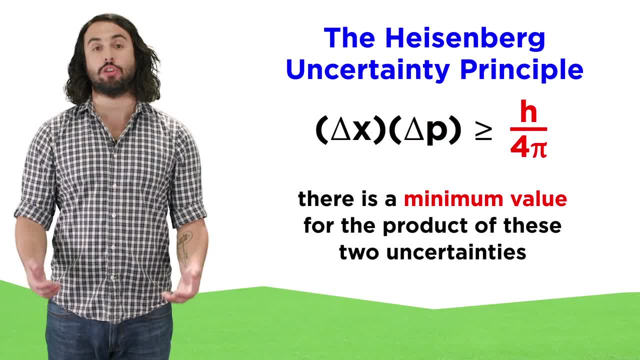 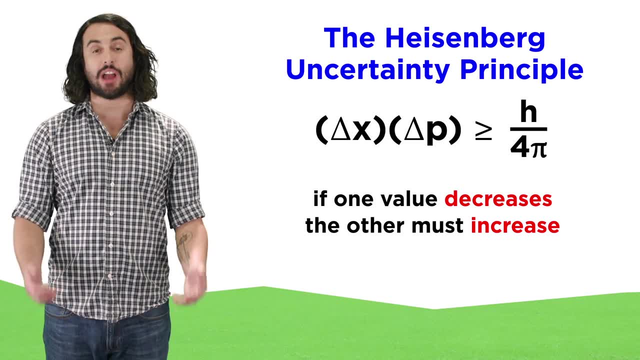 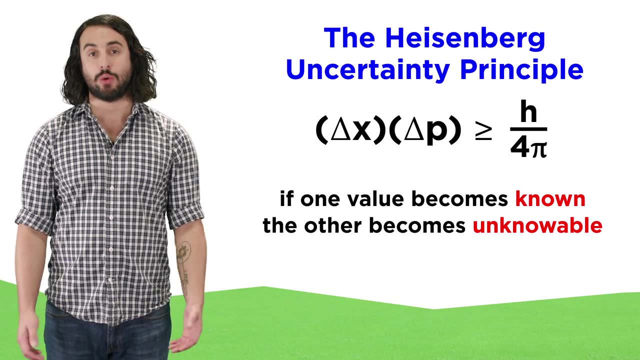 in position. Here, delta X represents the uncertainty in position, while delta P is the uncertainty in momentum, and their product must be greater than H over four pi. If the uncertainty in one parameter decreases, the uncertainty in the other must increase, and if one becomes known with total certainty, the other becomes unknowable. 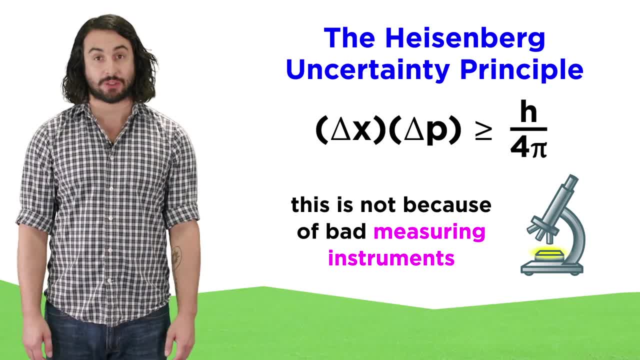 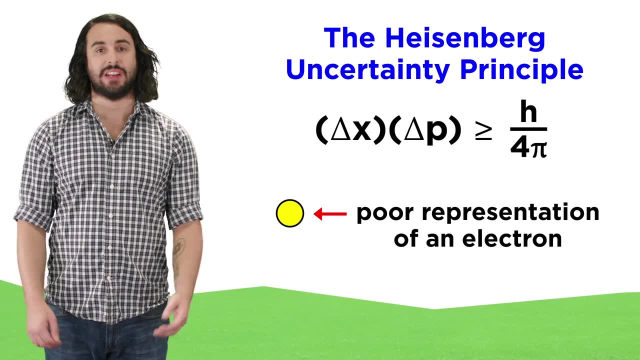 The important thing to realize is that this has nothing to do with our measuring instruments. This is a fundamental quality of matter. We can't reduce an electron to particle-like determinacy, As it is also a wave, as was demonstrated by the double-slit experiment. 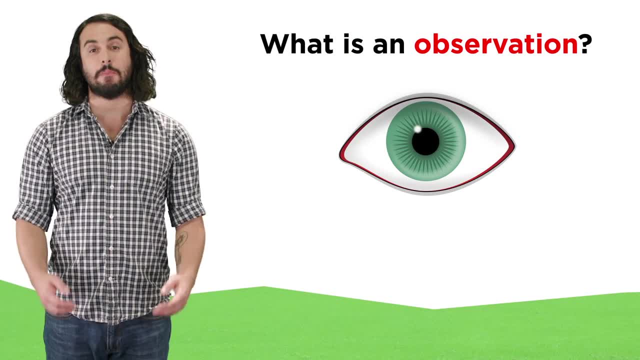 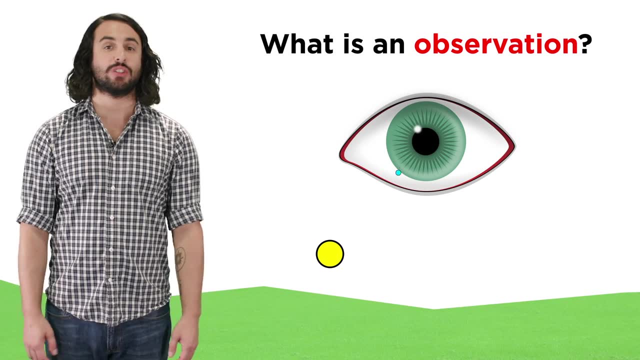 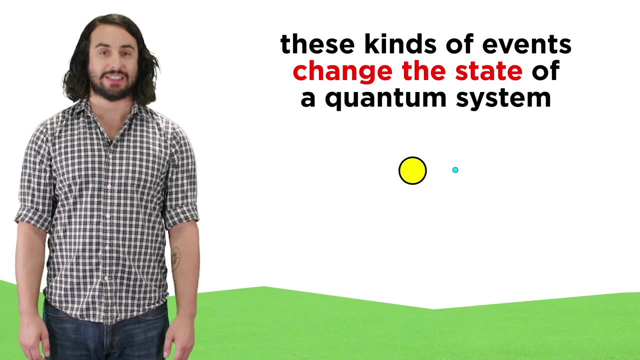 Furthermore, this forces us to examine what it is to make an observation, To know the location of an object, to see it, at least one photon must hit our eyeballs. But if a quantum system interacts with even just one photon such that it can be seen, 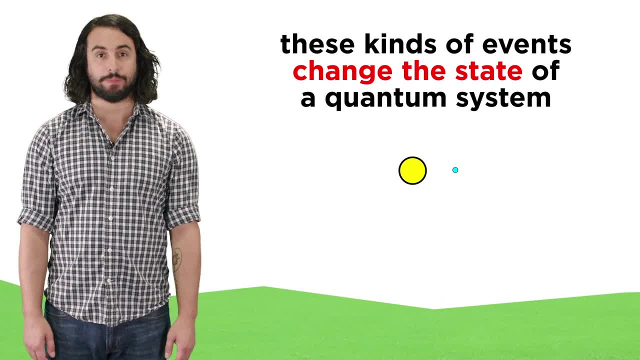 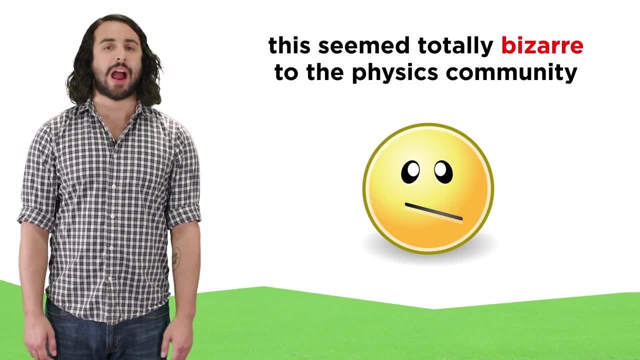 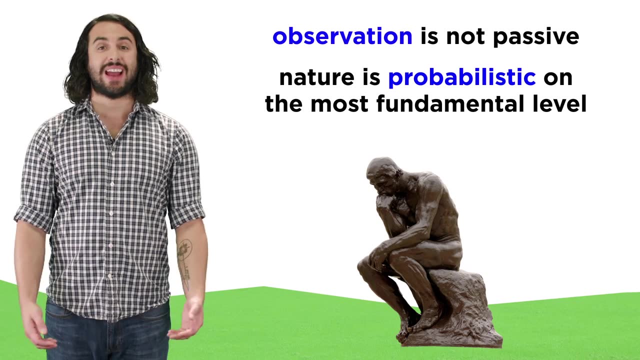 that interaction itself will alter the state of the system. so the seemingly innocent act of observation will change. The idea of observation has a concrete impact on the system. When this problem of measurement emerged, the scientific community was in total confusion. This notion and the idea that nature was not deterministic but rather probabilistic, 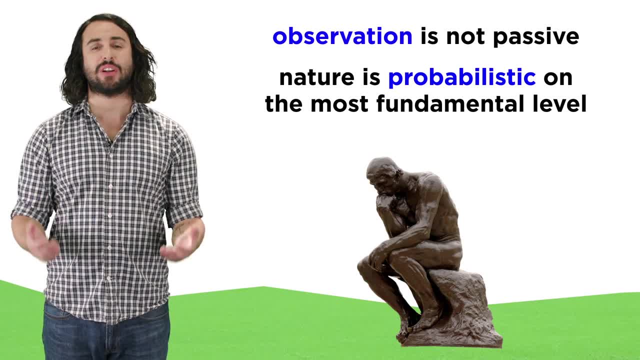 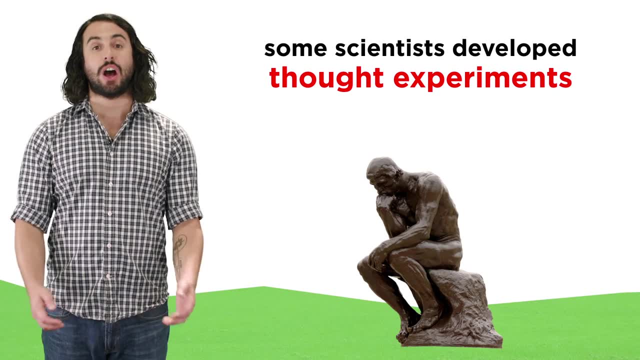 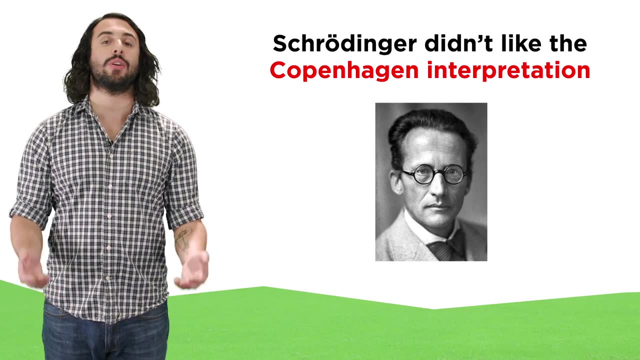 on the most fundamental level had incredible philosophical implications, and many scientists developed thought experiments to elucidate the absurdity of a probabilistic universe. The most famous of these thought experiments was developed by Schrödinger himself, as he could not accept the Copenhagen interpretation. 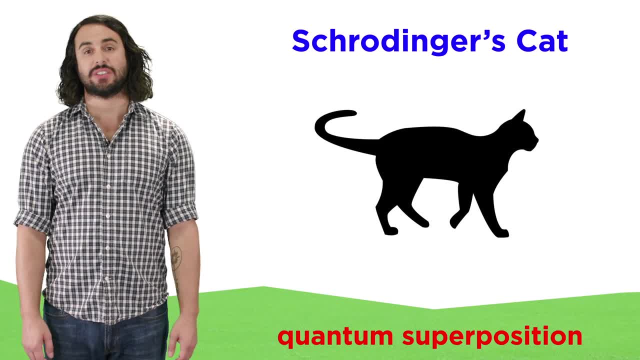 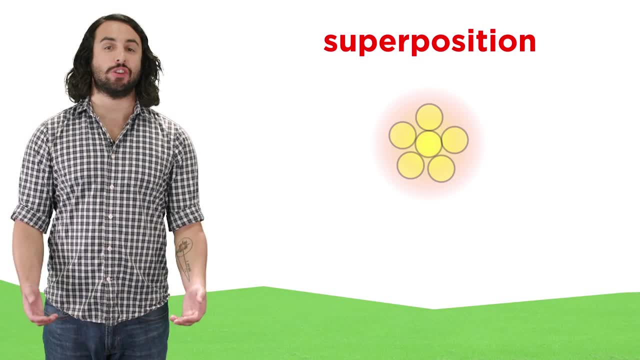 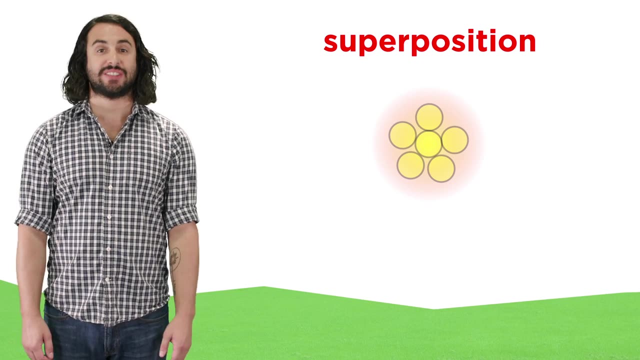 It is called Schrödinger's cat and it focuses on the bizarre concept of quantum superposition. The idea is that, if the Copenhagen interpretation is correct, a quantum system can exist in a number of different states and, until the system is observed, it exists in a superposition. 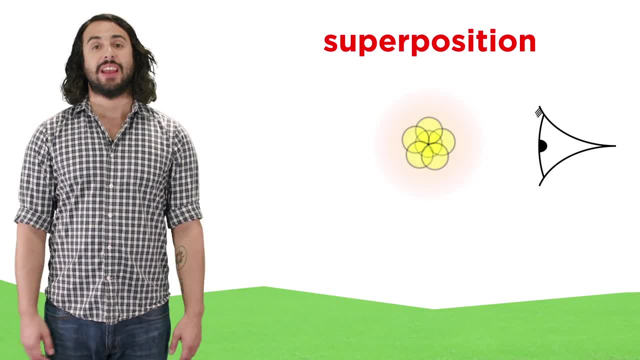 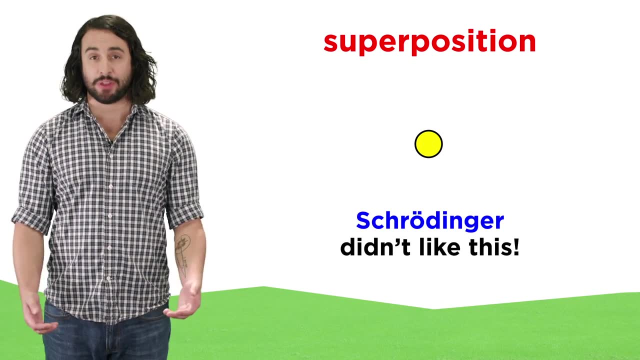 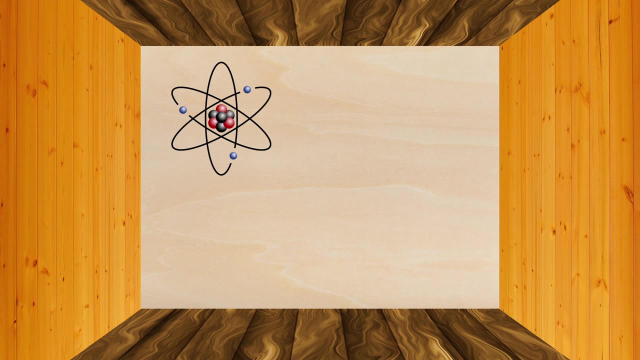 Once observed, it collapses into one of the definite states, according to its probability. Schrödinger did not like this and he came up with a paradox. He supposed that there was a box containing a single radioactive atom. At any given moment, this atom has the potential to decay, emitting a high-energy particle. 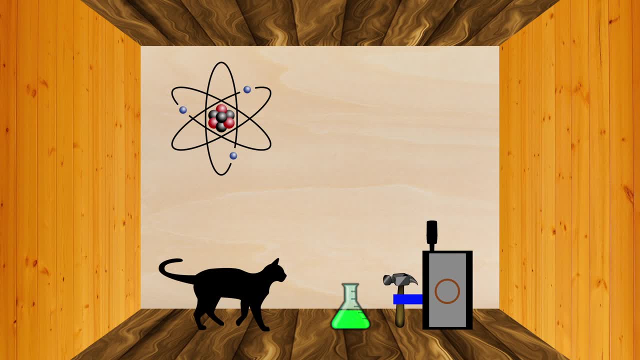 Inside the box there is also a cat, a flask of poison and a device with the ability to detect radiation. If the device detects that the atom has decayed, it will trigger a mechanism that breaks the flask of poison and the cat will die. 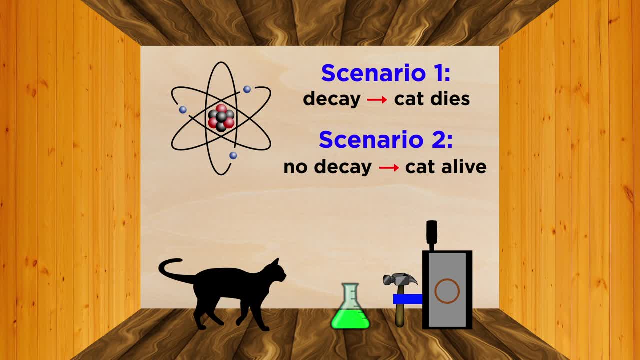 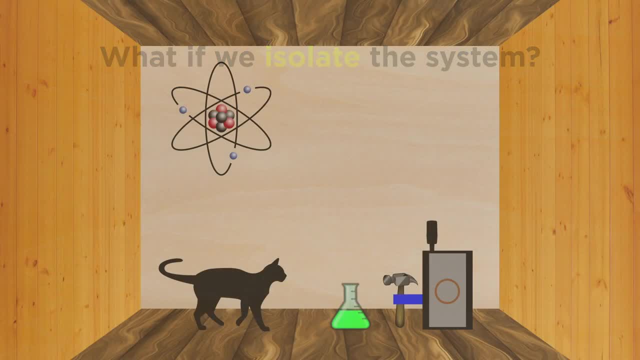 If it does not detect this, it won't and the cat will be alive. The problem arises when we isolate this system from observation. According to the Copenhagen interpretation, the atom is in a superposition of decaying and not decaying, which seems pretty abstract and harmless. 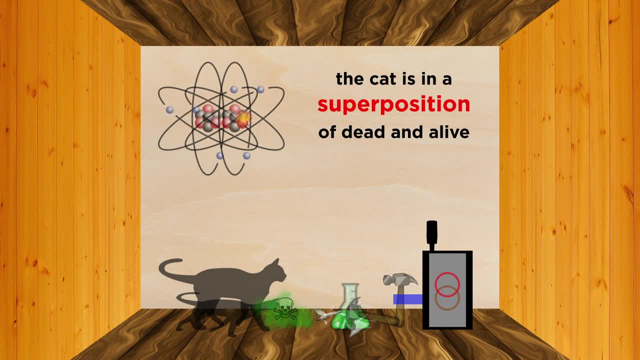 The problem is that the atom is in a superposition of decaying and not decaying, which seems pretty abstract and harmless, But because of the mechanism in the box that means that the cat must be in a superposition of dead and alive. 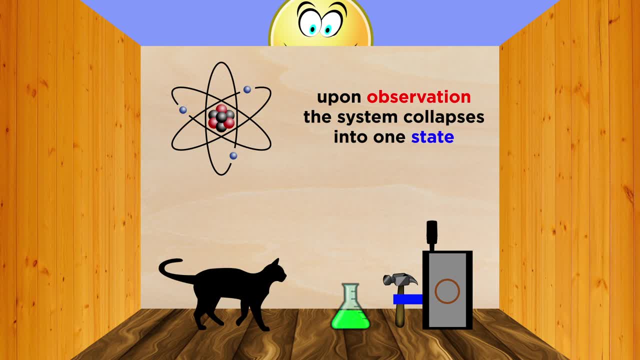 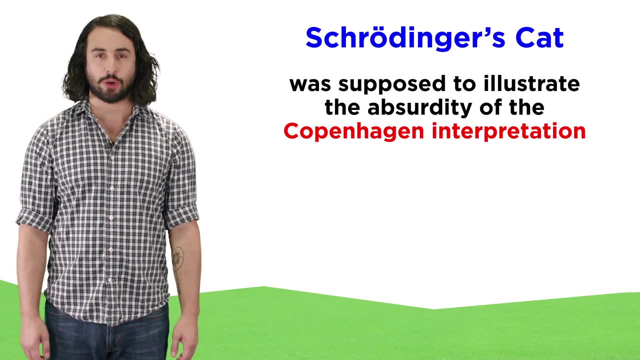 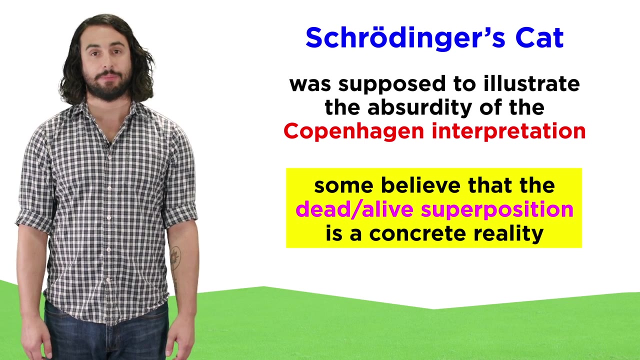 Only once you open the box and look inside will you observe the cat as being one or the other. Schrödinger meant for this paradox to discredit the Copenhagen interpretation, but there are many camps that believe that this dead-alive superposition is a concrete reality. 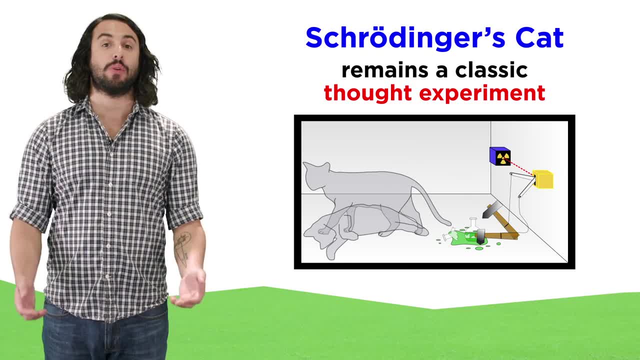 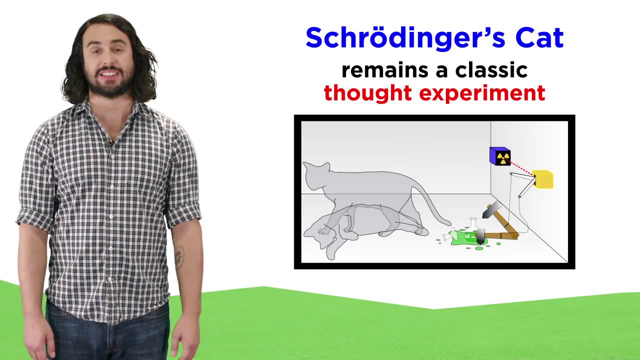 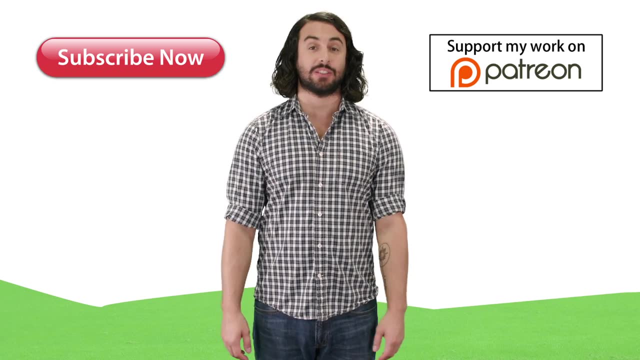 This thought experiment remains a classic And it is frequently referred to when comparing different interpretations of quantum mechanics. But enough about cats, let's finish up with Heisenberg. Thanks for watching, guys. Subscribe to my channel for more tutorials. support me on Patreon so I can keep making. 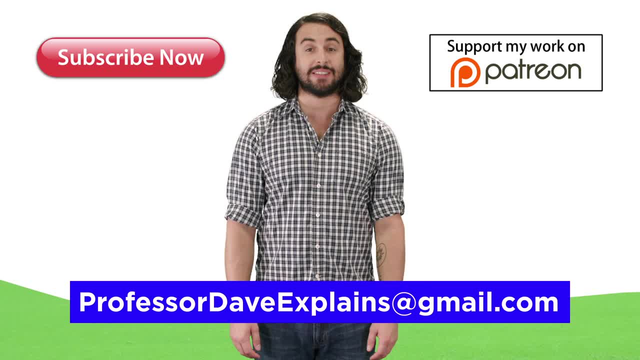 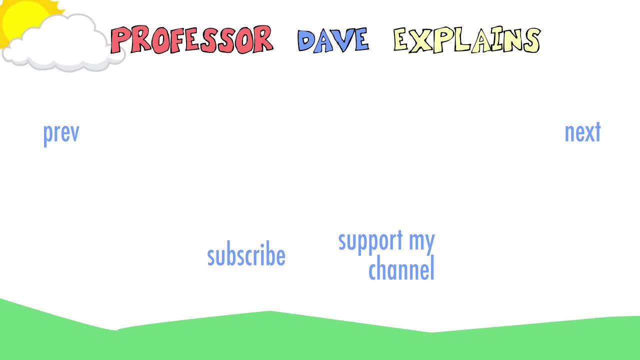 content and, as always, feel free to email me professordaveexplains at gmailcom. I'll see you in the next one. Bye.